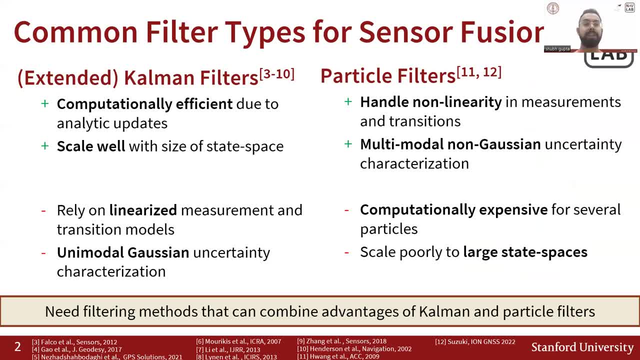 filters and their family, such as the extended Kalman filters, are computationally efficient due to performing analytic updates as well as scale well with the size of the state space. However, they rely on linearized measurement and transition. The Bayesian filters have been used for sensor fusion, which can characterize uncertainty. 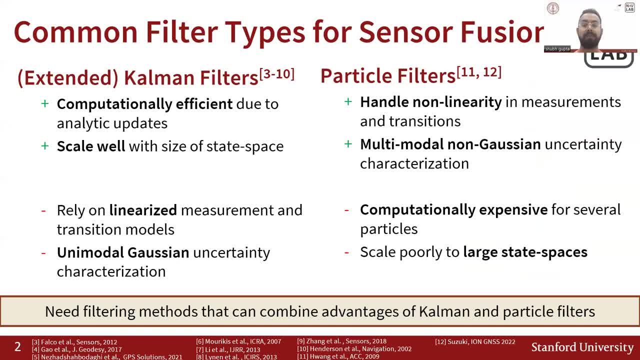 using the unimodal Gaussian, which has limited performance in the real world. On the other hand, particle filters can handle nonlinearity in measurement and transition as well as characterize a multi-modal and non-Gaussian uncertainty. However, particle filters are computationally expensive to run, especially when the number of particles is. 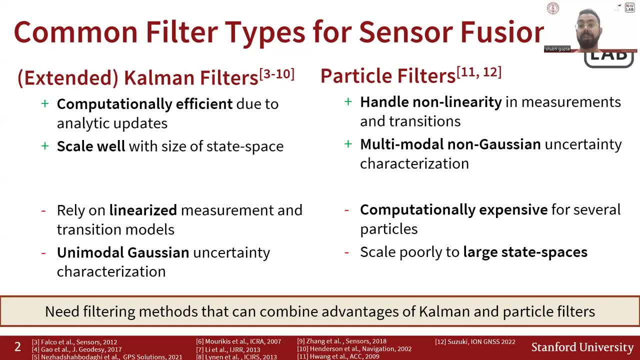 high and scale poorly to large state spaces, which is important So they can be used for, which is usually a requirement in most real-world applications. So there is a need for filtering methods that can combine the advantages of both Kalman and particle. 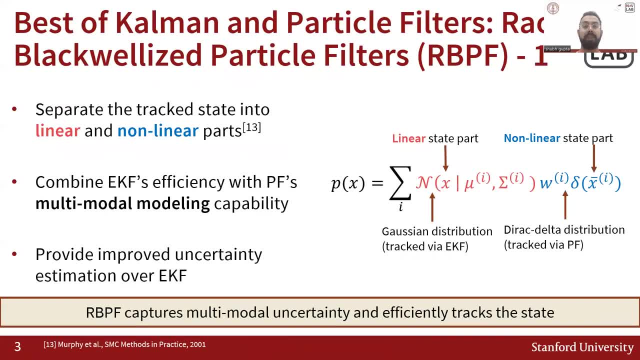 filters. Rao-blackballized particle filters, or RBPF, are one such types of filters that operate by separating the tracked state into linear and nonlinear parts. The linear part is tracked efficiently as a Gaussian distribution using an extended Kalman filter, while the nonlinear part is tracked using a particle filter. 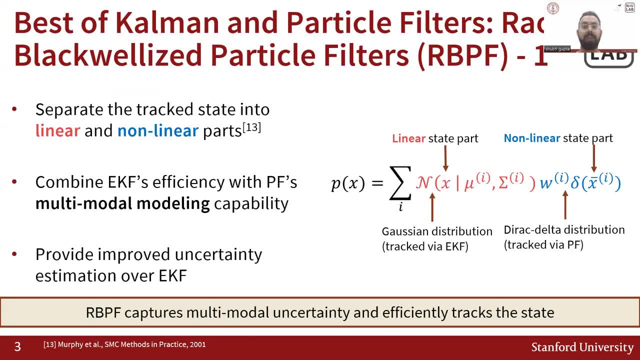 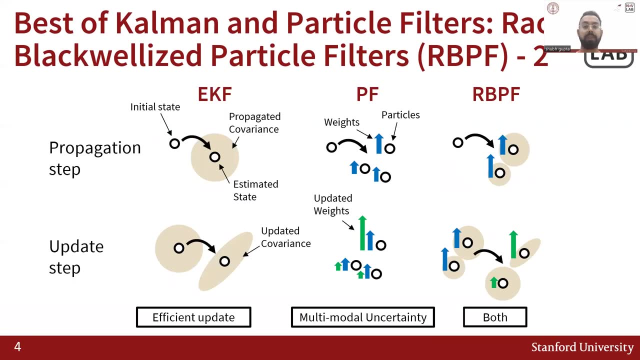 to better model the uncertainty. Hence Rao-blackballized particle filters combine an EKF's efficiency with a particle filter's multimodal modeling capability and provide improved uncertainty estimation over pure EKF. Here is a visualization to give a sense of how an RBPF combines. 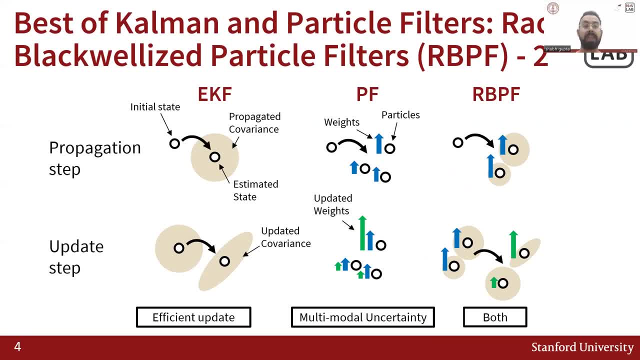 both of these, looking at the propagation and update steps of different filters. An EKF efficiently propagates and updates the estimated state, as well as covariance as a Gaussian distribution. Compared to that, a particle filter updates the weights associated with a discrete set of particles, which better characterizes. 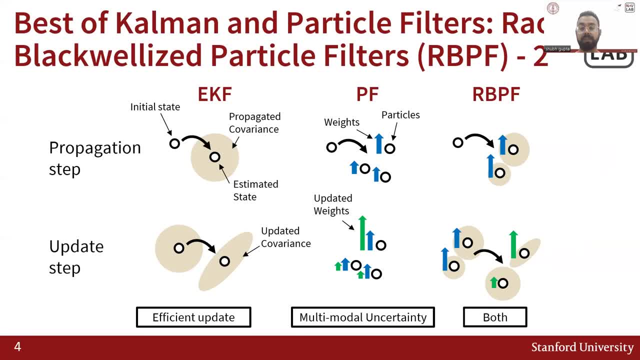 the multimodal uncertainty. Compared to both of these two, an RBPF both efficiently updates the weights associated with different particles and efficiently updates the parametric uncertainty. Here is an example of a Gaussian distribution that is also associated with each particle and has both the advantages. 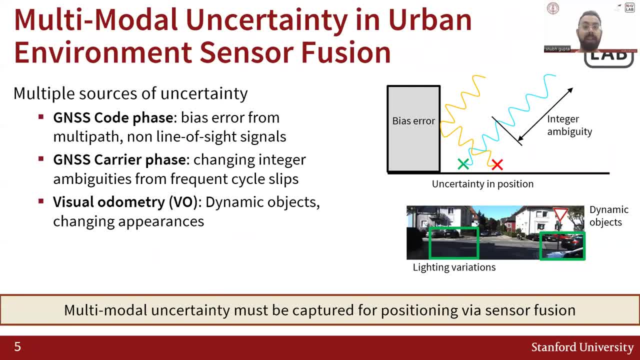 And this ability to be able to characterize a multimodal uncertainty is important for sensor fusion in urban environments where there are multiple sources of uncertainty present from the sensors. For example, in GNSS code phase the uncertainty arises from bias errors, from multipath and non-line. 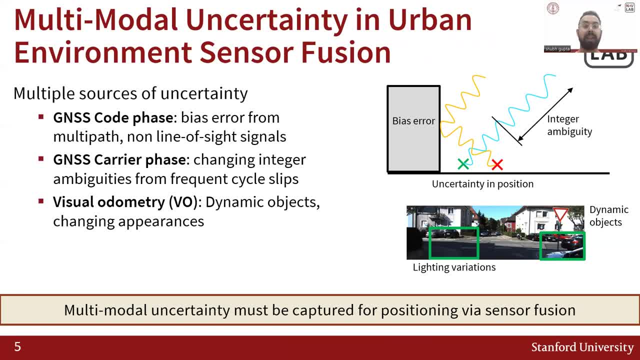 of sight signals, But carrier phase. it is from the changing values of integer ambiguities, from frequent cycle slips, And for visual odometry it is from dynamic objects as well as changing appearances in the environment. So multimodal uncertainty must be captured for positioning. 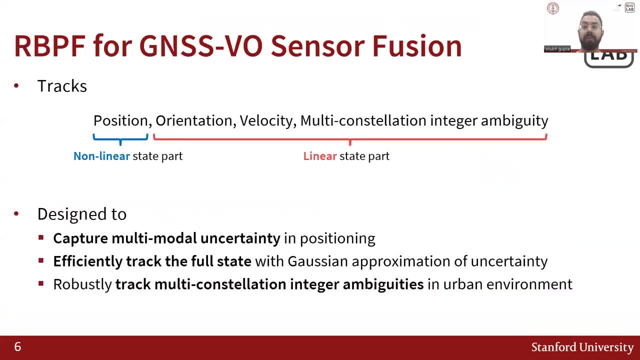 via sensor fusion, And this is why we use an RBPF for developing a GNSS view sensor fusion approach. In this work, we track, using the RBPF, a state that comprises of the position, orientation, velocity and the distribution. The position is tracked as the non-linear state part. 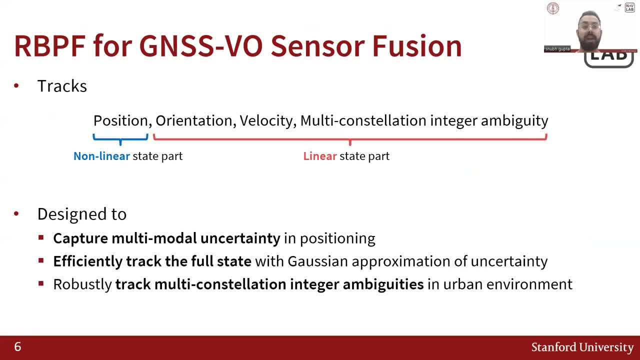 in the RBPF, while the rest of the state components are tracked efficiently as the linear part. Hence our RBPF, designed this way, is able to capture multimodal uncertainty in positioning, efficiently track the full state using Gaussian approximations and robustly tracks multi-constellation integer. 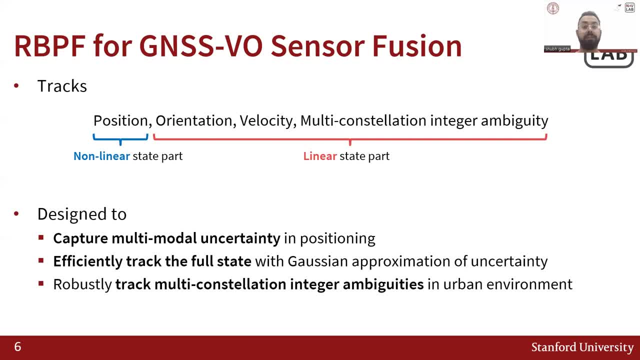 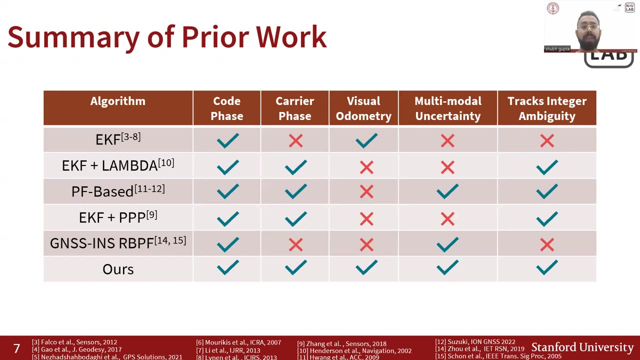 ambiguities in urban environments. So in this work we are able to capture multi-modal uncertainty in positioning, efficiently track the full state using Gaussian approximations and robustly tracks multi-constellation integer ambiguities in urban environments. Here is a summary of prior work on filtering for sensor fusion. 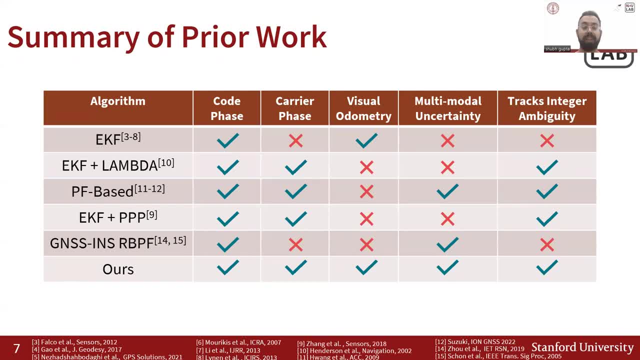 We categorized these works based on their support for code phase measurements, carrier phase measurements and visual geometry, as well as whether they characterize a multimodal uncertainty or track the integer ambiguity. To the best of our knowledge, our RBPF-based approach is the first that satisfies all of these criteria. 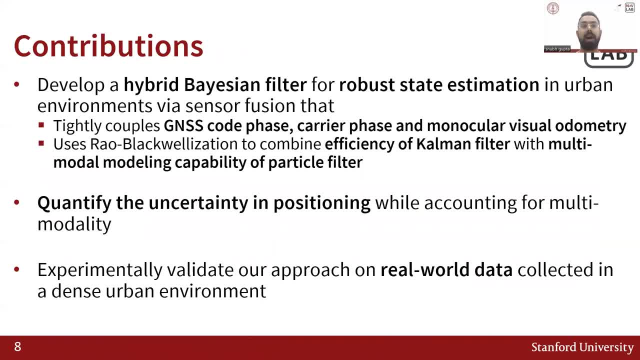 Contributions from this work are as follows: We develop a hybrid Bayesian filter for robust state estimation in urban environments via sensor fusion that couples tightly GNSS code phase, carrier phase and monocular visual odometry measurements, And for that it uses raw black visualization. 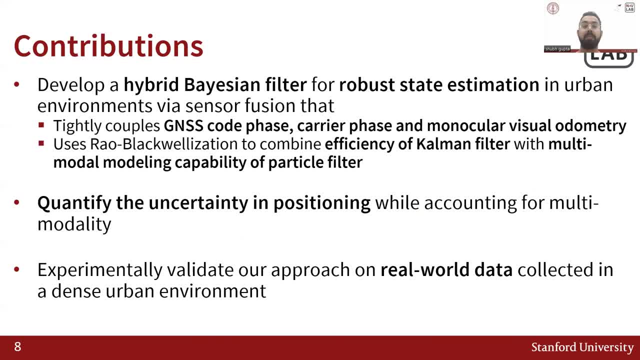 to combine the efficiency of carbon filters with multimodal modeling capability of a particle filter and utilizes that to quantify the uncertainty in positioning, while accounting for multimodality. We also experimentally validate our approach on real-world data that is collected in a dense urban environment. 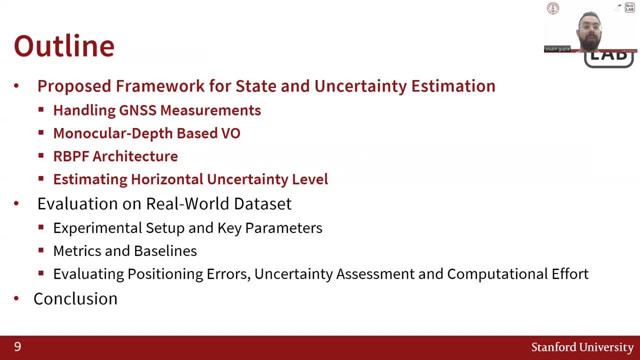 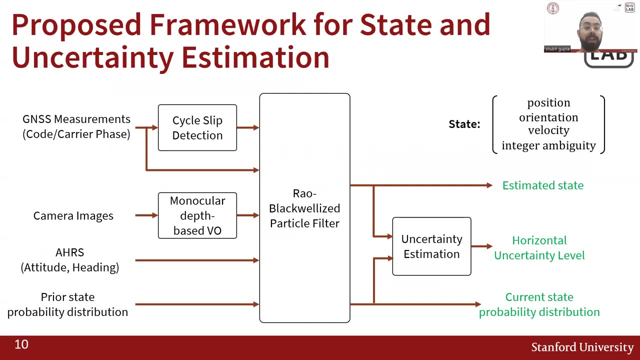 Here is the outline for our talk. I will talk about our proposed framework for state and uncertainty estimation and each of the components involved in detail. Next, I will talk about our evaluation on real-world data set and finally conclude. So here is the architecture. 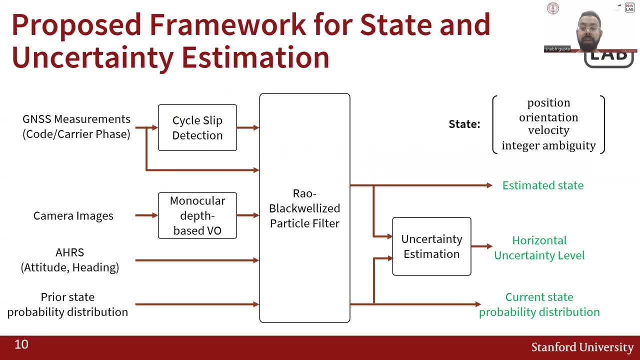 for our proposed framework for state and uncertainty estimation. We start from processing the measurements, including GNSS code and carrier phase measurements to detect cycle slips, as well as camera images to compute visual odometry based on monocular depth. Next, we combine these with the attitude. 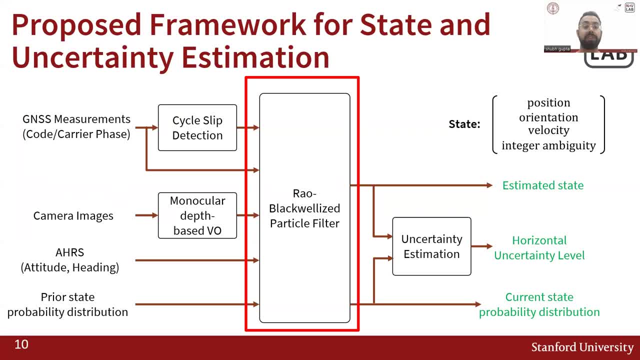 and heading measurements from AHRS and the prior state probability distribution and pass them to the raw black analyzed particle filter that assimilates this information to produce the estimated state as well as the current state probability distribution. We also use this information in an uncertainty estimation module. 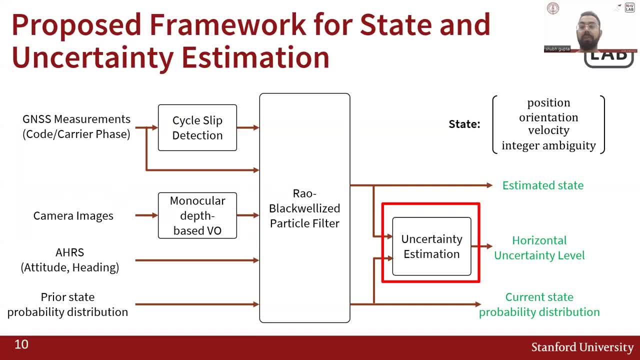 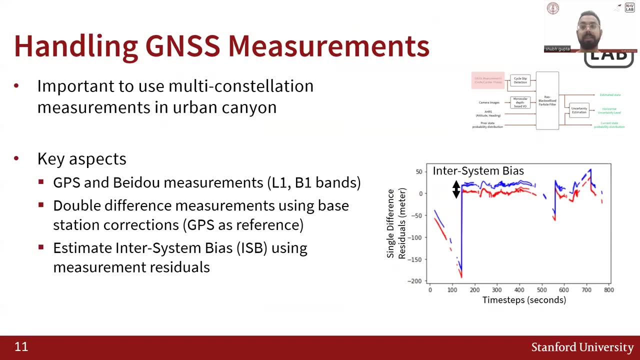 to determine or quantify the uncertainty using the metric of horizontal uncertainty level. I will next talk about our measurement processing process For handling GNSS measurements. an important consideration in urban environments is to account for limited satellite visibility, So it is important to use multi-constellation measurements. 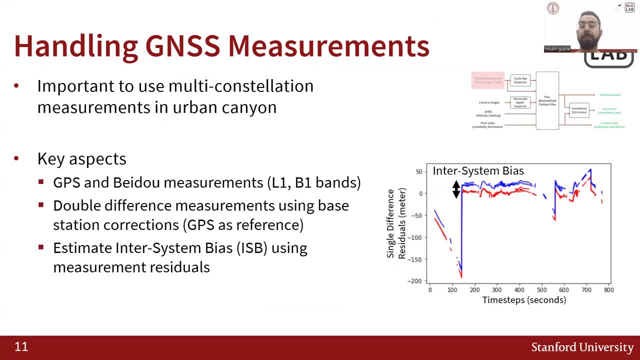 in these urban canyons, which our filtering approach has support for. The key aspects of our multi-constellation support are that we account for both GPS and PADO measurements from L1 and B1 bands, so single frequency measurements and compute double difference measurements. 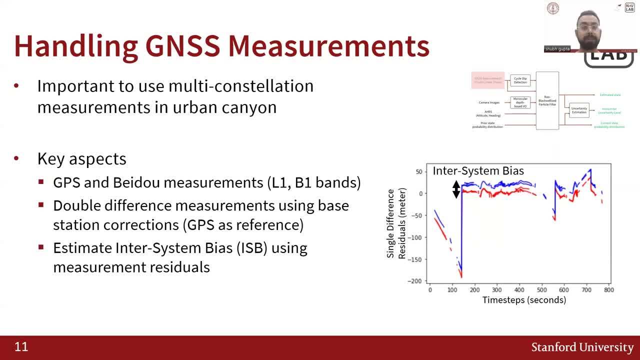 by using PADES, station connections and GPS as a reference. Then, to account for the multi-constellation setup, we pre-estimate the inter-system bias using measurement residuals, as can be seen from the figure on right, and correct the measurements based on that. 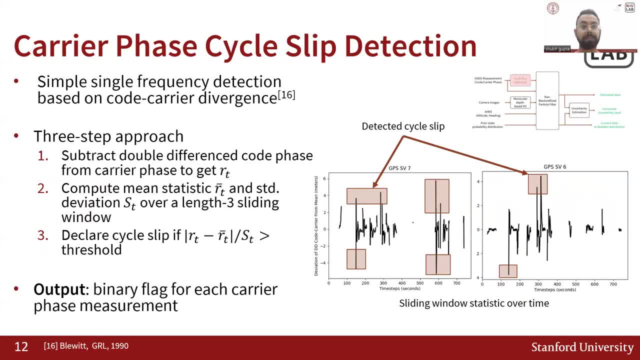 before inputting them to the filter. We also perform cycle slip detection for carrier phase measurements, since these are frequent in urban environments, And for that we use a simple single frequency detection strategy that is based on code carrier divergence. Our strategy has three steps. 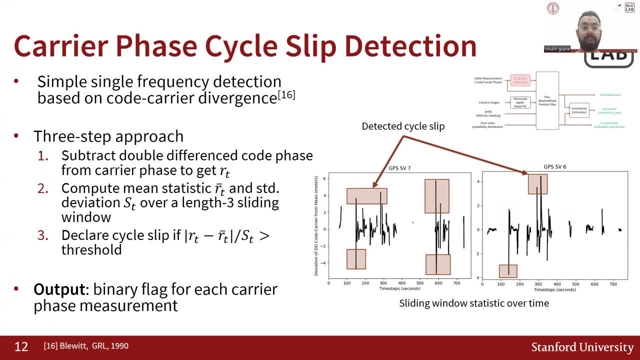 where we first subtract the double-differenced code phase and carrier phase measurements to get a divergence value for each type And from that we compute the mean statistic as well as the standard deviation over length 3 sliding windows. Finally, we declare a cycle slip. 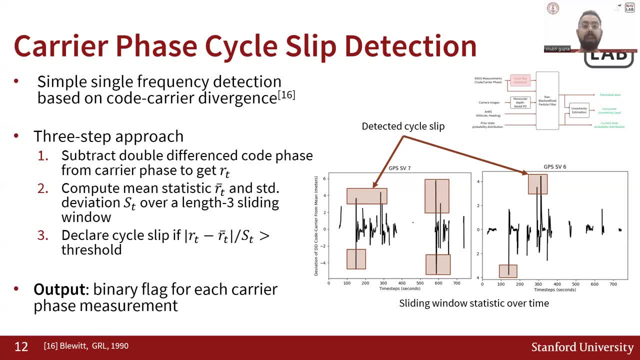 as the value of the statistic exceeds a threshold value, and output a binary flag for each measurement, as can be seen from the figure on the right. Finally, we declare a cycle slip, as the value of the statistic exceeds a threshold value, and output a binary flag for each measurement. 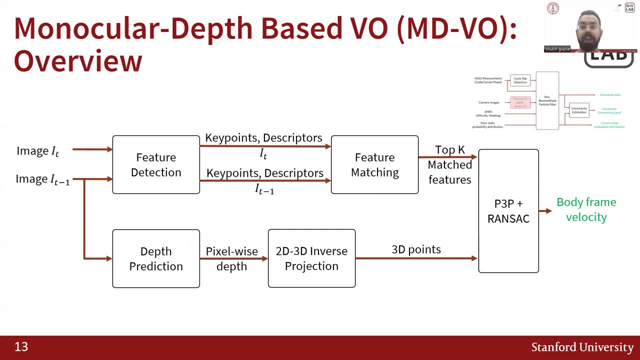 as can be seen from the figure on the right. Next, I will move on to describing our pipeline for processing camera images to generate the visual odometry values as the body frame velocities, Starting from the camera image acquired at the current time as well as the previous time. 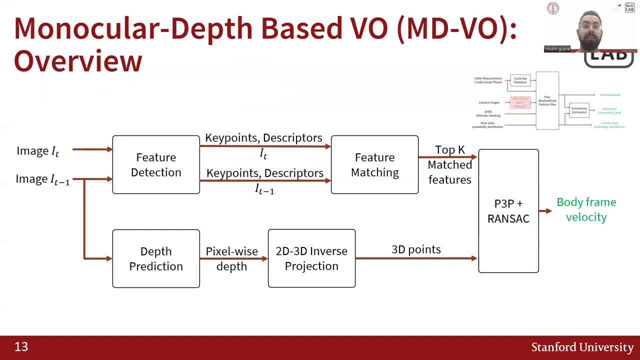 we detect features over it to identify key points as well as descriptors. Then we match these features and identify the top k matched features which are to be used for the subsequent part. Parallel to this, we use the previous time camera image to output a pixel-wise depth. 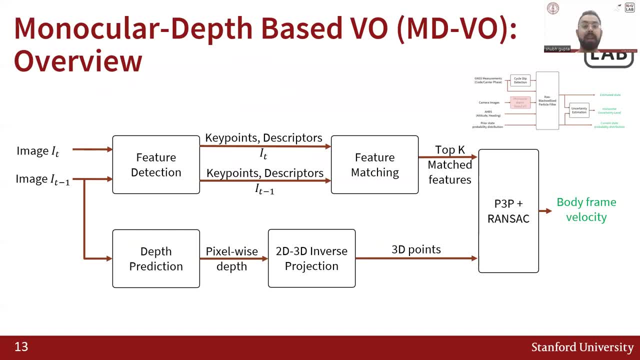 using a depth prediction module which I will describe in the next slide, And using this pixel-wise depth, we project the matched features to 3D coordinates and perform 2D to 3D matching using P3P plus RANSAC to output the final body frame velocity. 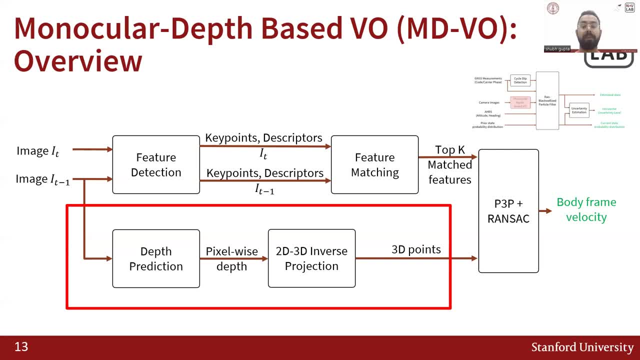 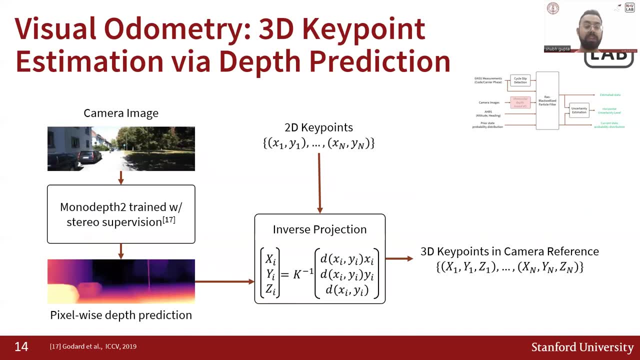 Next I will talk about this process of predicting depth and projecting the key points to 3D coordinates. To do that, we start from the camera image that is, the previous time camera image and pass that through a neural network that is trained for predicting depth. 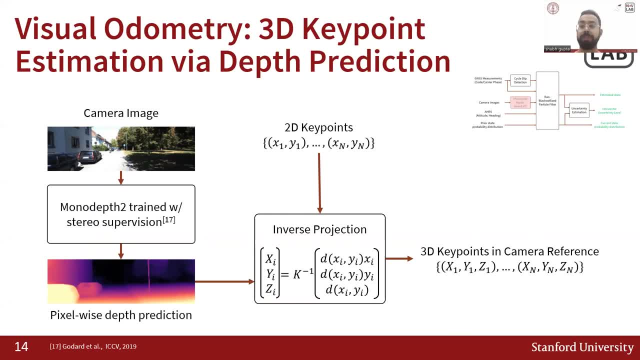 For this we use MonoDepth2 that is trained with stereo supervision. We use a neural network for this task because generating pixel-wise depth from a monocular camera image is inherently an ill-posed task. However, previous research has shown that a neural network is able to perform this task. 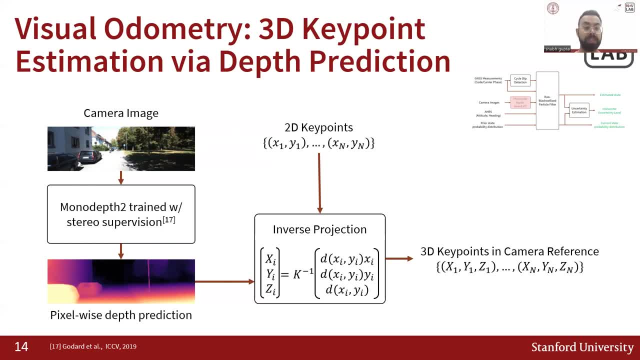 using heuristics fairly well, Of using the pixel-wise depth predictions from the neural network. we project the 2D key points that we detected on the camera image using the camera projection matrix and inverse projection into 3D key points that are in the camera reference wave. 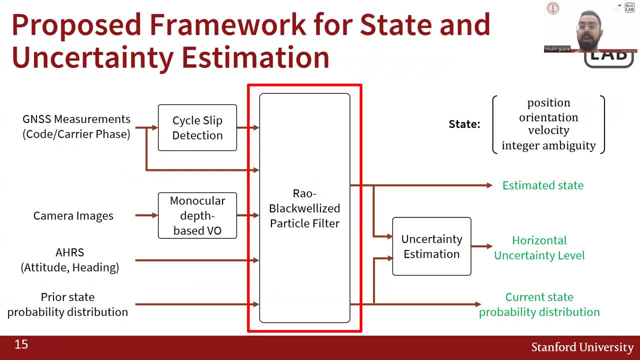 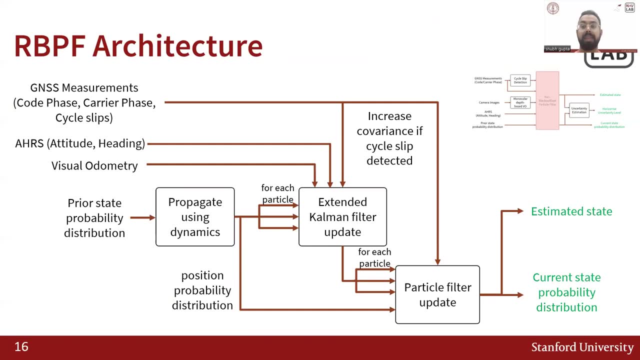 Now I will move on to our Rao-Blackwellized particle filter that assimilates all the information from the different measurements, as well as the previous probability distribution. Here is our RBPF architecture that uses all this information to estimate the state, as well as update the state probability distribution. 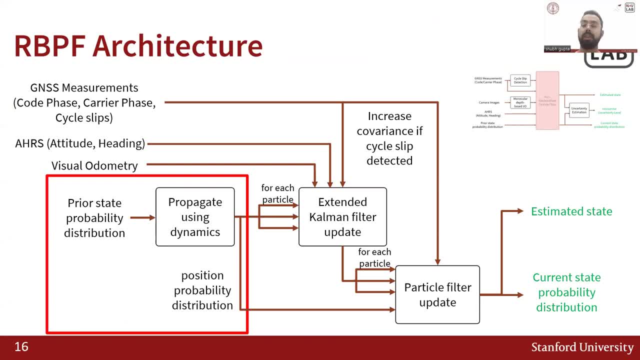 First we start from the prior state probability distribution, which is propagated using dynamics and is passed to the extended Kalman filter. Along with that, a component of this propagated state probability distribution, which is specifically associated with the position part, is passed to a particle filter as well. 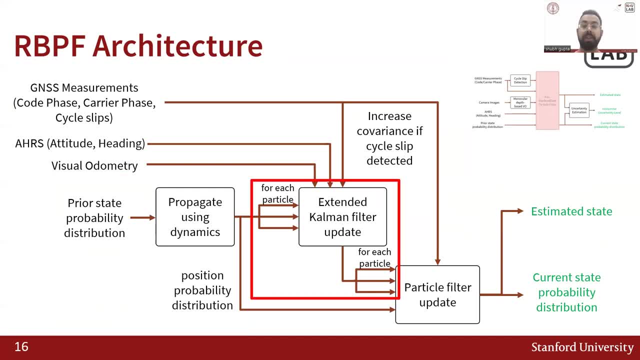 Using the propagated state probability distribution that is passed to the filter, as well as the measurements and features detected from the previous steps. we apply an extended Kalman filter update to compute the updated state probability distribution And we perform this step for each particle, as is done in the Rao-Blackwellized particle filter. 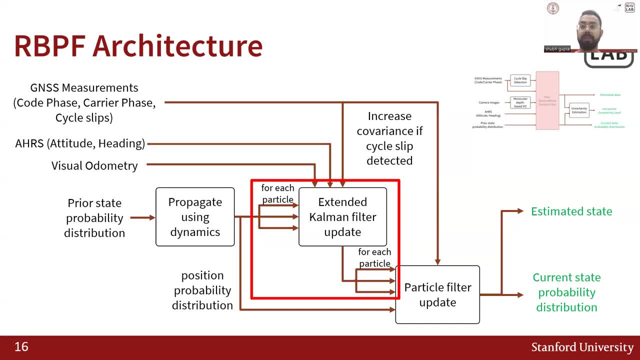 Within this extended Kalman filter, the covariance values are scaled whenever a cycle slip is detected in the previous module. These updated state estimates are passed to the particle filter along with the position probability distribution from the propagation step, and the particle filter then performs its own update step. 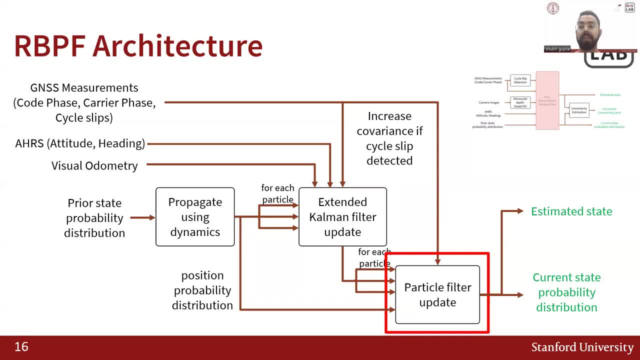 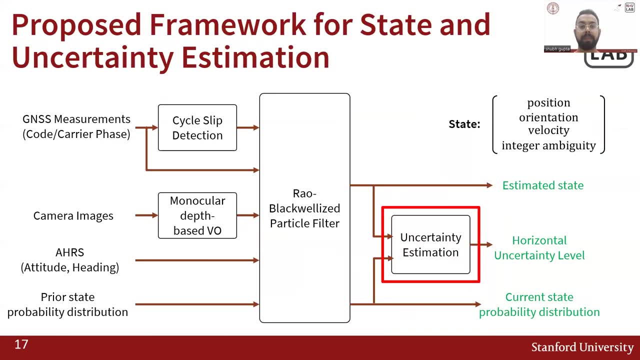 using the GNSS measurements. In this step we compute the estimated state probability distribution as well as the current state probability distribution. So now that I have gone over our Rao-Blackwellized particle filter to generate the estimated state and the state probability distribution, 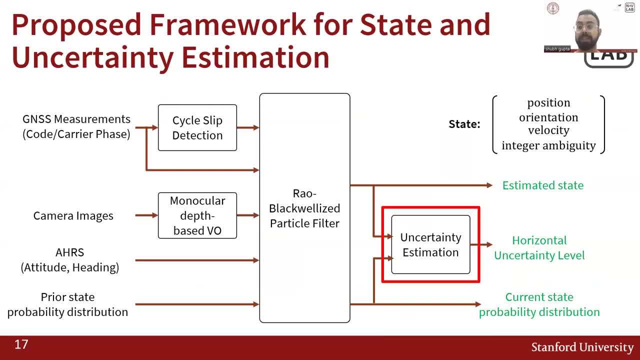 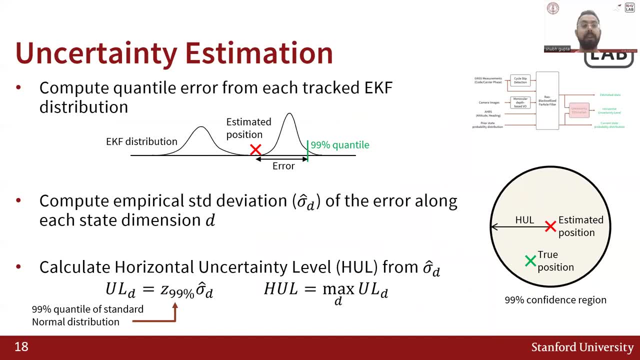 I will now talk about the uncertainty estimation process from this. So our uncertainty estimation process occurs in three steps. First, we compute quantile errors from each of the tracked extended Kalman filter distributions And these errors are computed relative to the estimated position, as can be seen in the first figure. 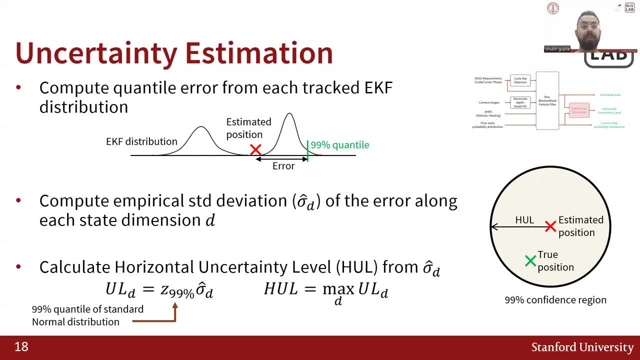 Using these quantile errors, we compute an empirical standard deviation of the error along each of the state dimensions, which are specifically the north and east dimensions. From this empirical standard deviation we compute the 99% quantile, using the standard normal distribution to generate and take the maximum. 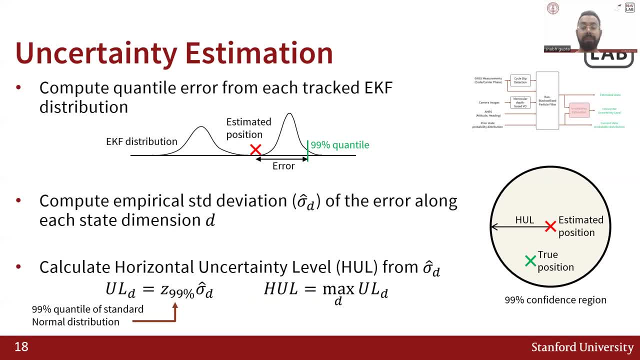 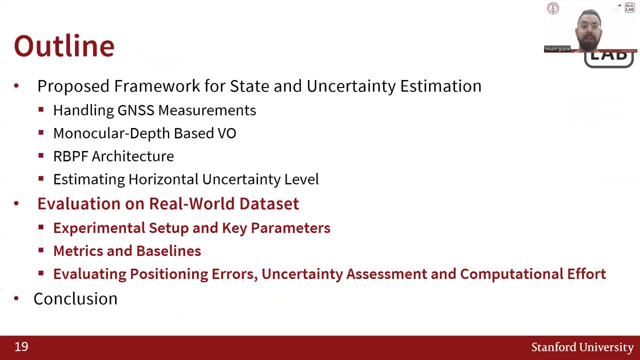 along both the directions to compute the overall horizontal uncertainty levels. The figure on the right visualizes the horizontal uncertainty levels, which describe a 99% confidence region around the estimated position that bounds the true position. So now that I have described our framework, 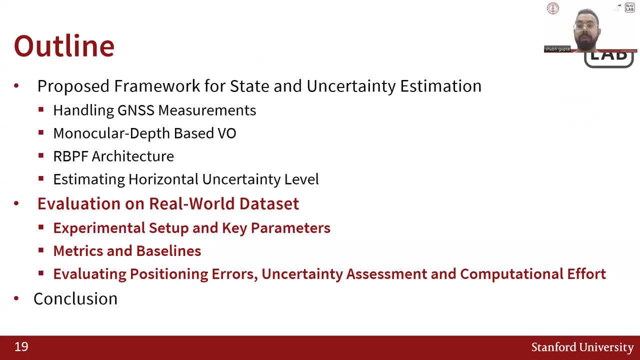 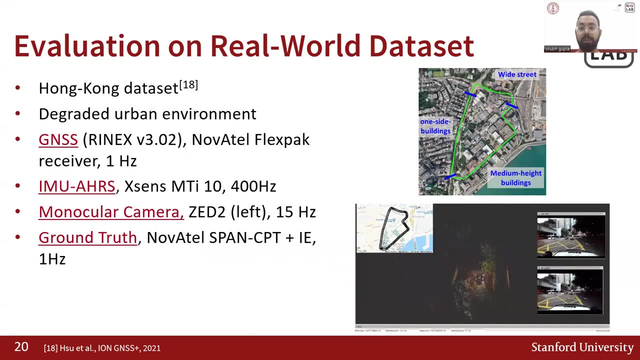 I will move on to our process of evaluation using a real-world dataset. We use the Hong Kong dataset, which is collected in a degraded urban environment, for our evaluations, And the trajectory, as well as some pictures, can be seen on the right. The dataset consists of a: 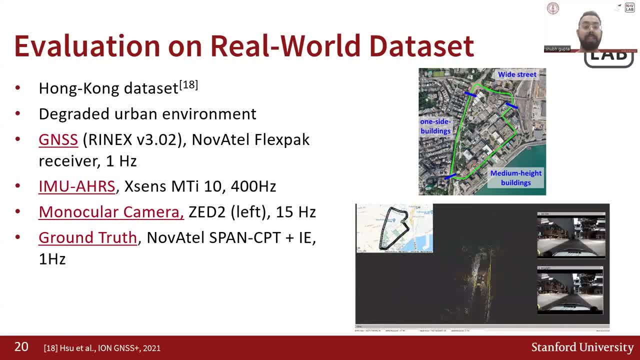 GNSS receiver, which is a Novotel FlexPAC receiver available at 1 Hz, as well as an IMU AHRS system, which is the Xsense MTI-10 that is available at 400 Hz. We also use monocular camera data. 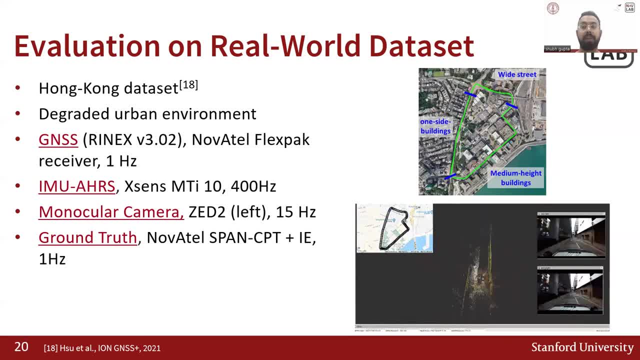 from the dataset, for which we use the left camera frame of the available Z2 camera, that is available at 15 Hz. And for ground truth, the dataset uses Novotel SPAN-CPT, with some corrections that is available at 1 Hz. 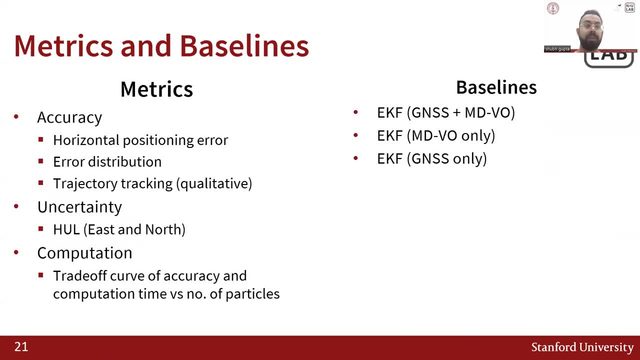 We evaluate our approach on this dataset for its ability to be able to perform positioning with good accuracy, perform uncertainty estimation and also not take too much of compute time. For accuracy we use the metrics of horizontal positioning error, the error distribution, as well as a qualitative view. 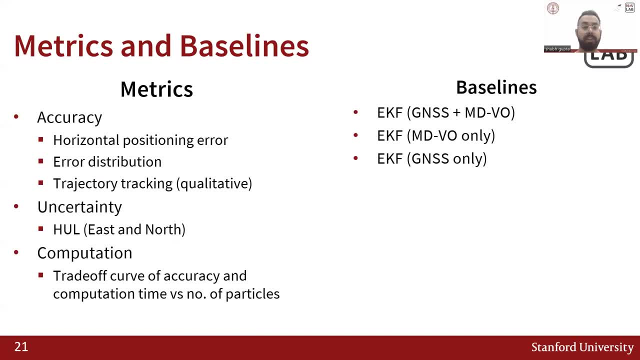 of the trajectory tracking. For uncertainty, we evaluate the horizontal uncertainty levels that are computed along the east and north direction, And for computation we use the trade-off curves of accuracy and computation and compare them as the number of particles is increased For our baselines for evaluating. 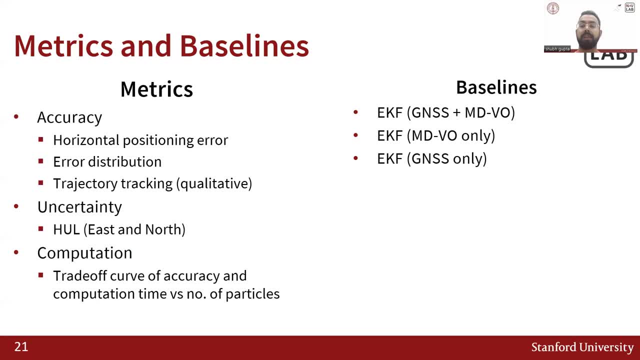 for evaluating these metrics. we use EKFs that are used in GNSS only, MDVO only, and both GNSS and MDVO settings. We do not explicitly show comparisons with the particle filter, because we observe from our experiments that the particle filter diverges. 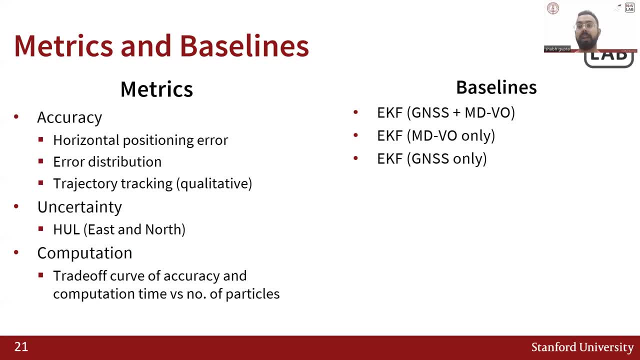 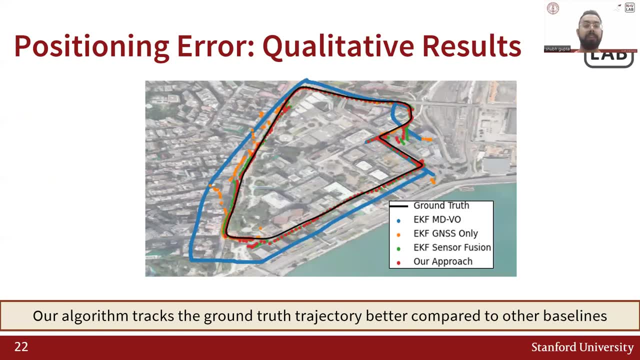 for the size of the state space as ours and therefore is not a good baseline. So here are our first set of qualitative results. on the positioning error, As can be seen from the trajectory tracks, our algorithm is able to track the ground truth trajectory better. 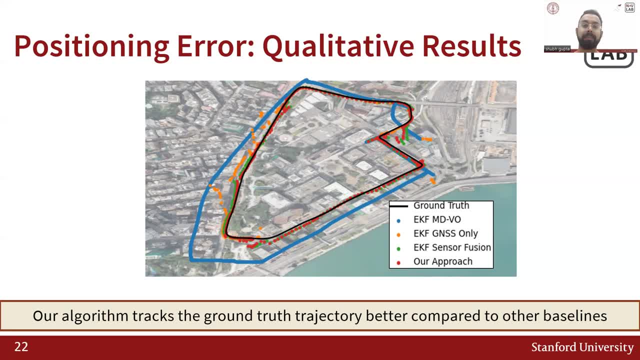 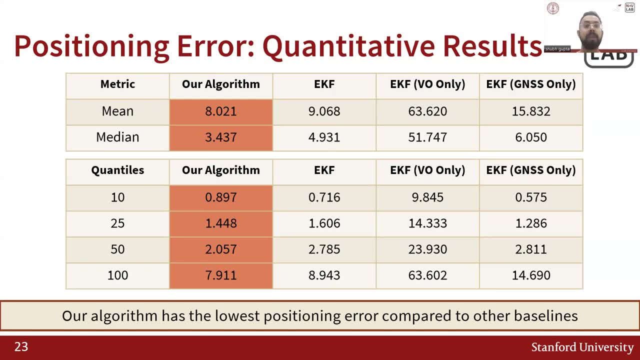 compared to other baselines. Next are the quantitative results that show the same result. numerically, Our algorithm achieves the lowest mean and median errors compared to all the baselines and also low values of errors in all the high values of contacts. Therefore, our algorithm has 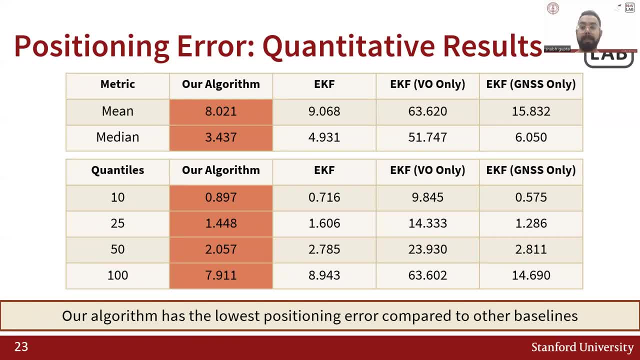 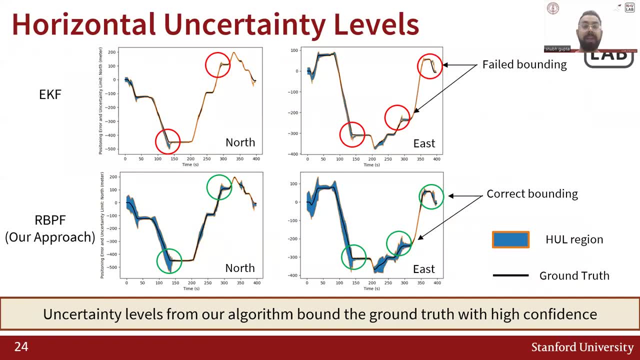 the lowest positioning error compared to other baselines. We also evaluate the ability of our algorithm to estimate the uncertainty, and for that we compare against an EKF that uses both GNSS and MDVO, As can be seen from the top plot, the horizontal uncertainty levels. 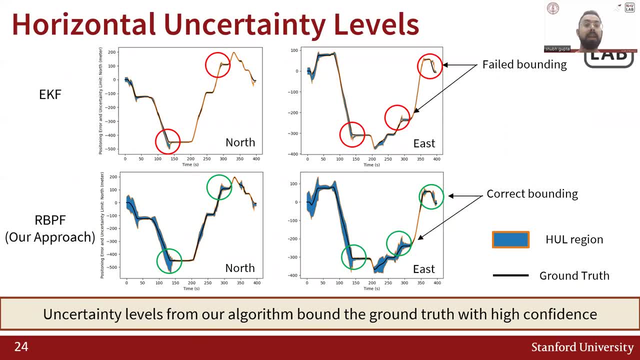 computed using the EKF covariance, only fail to properly bound the positioning error at multiple spots in the trajectory. Compared to that, our RBPF-based approach produces more conservative bounds, but they are able to bound the positioning errors successfully for most part of the trajectory. 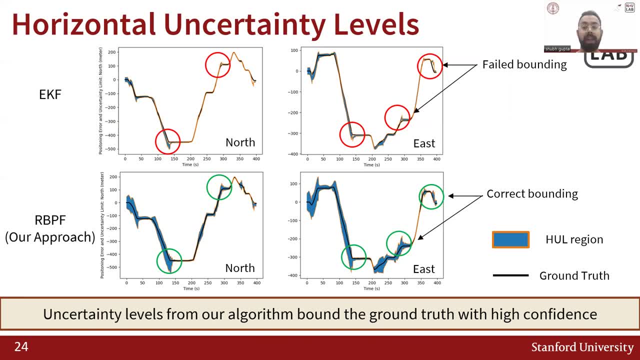 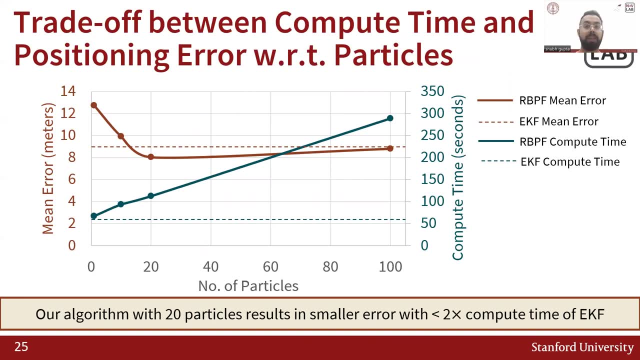 Therefore the uncertainty levels from our algorithm are more reliable. Finally, we also compare a trade-off between the compute time and the positioning error as the number of particles is increased. We also plot the EKF mean error and EKF compute time on the same plot for reference.